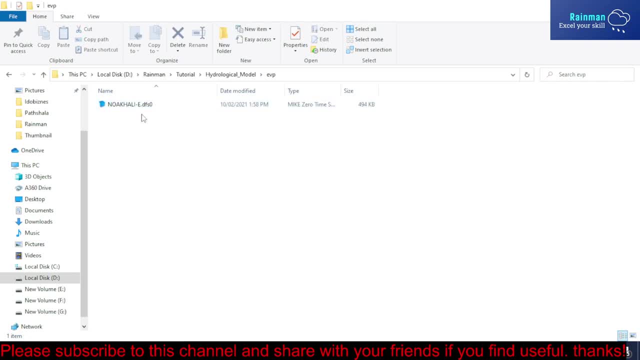 you have to keep the evaporation time series. So in this area, for which area you are doing the hydrological model and how many stations, how many evaporation stations actually govern there, You must have these evaporation data and you have to have the time series of evaporation and place the time. 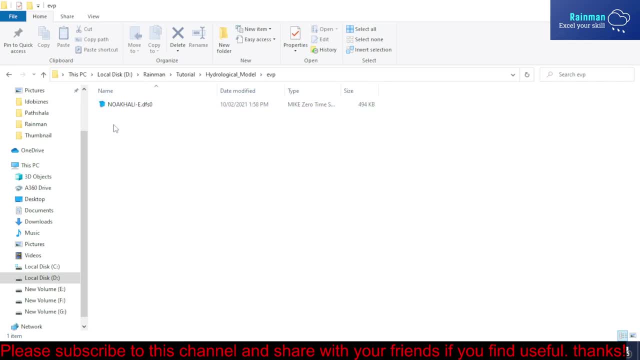 series file, that is a DFSO file in this folder. I have only one evaporation station which dominates my hydrological area, So only one time series of evaporation I have kept here. So how will you make a DFSO file or time series? I have prepared a. 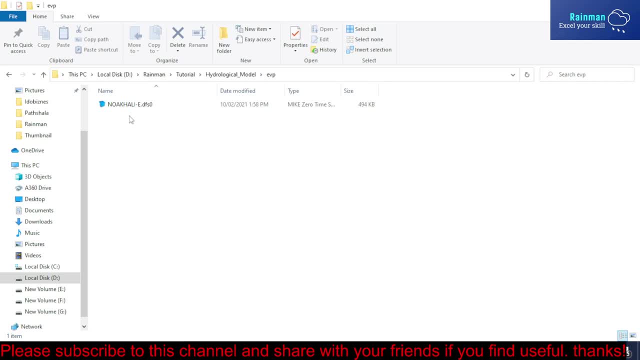 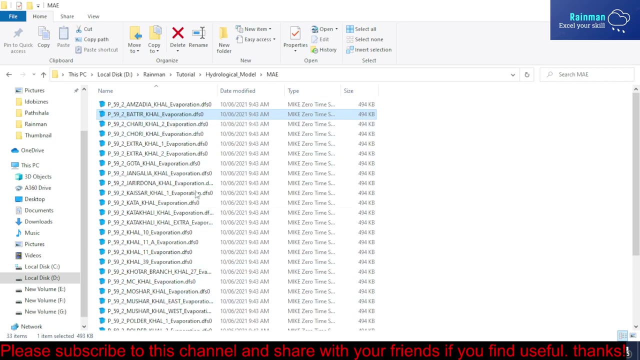 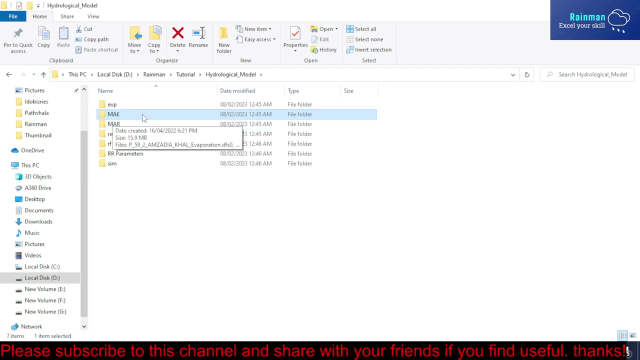 tutorial on this and you can watch this tutorial in my channel. so this is evaporation data and this is mae. actually, these, these files, all the files have been created. when you simulate the model, nothing to do it with these files. this is mae. that is mean aerial evaporation. 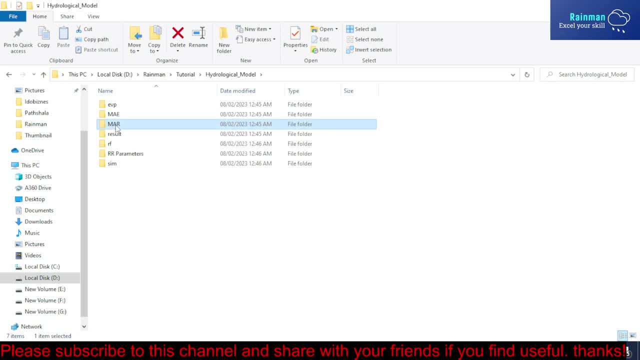 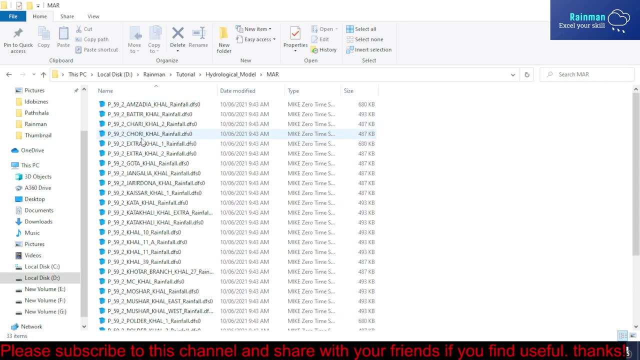 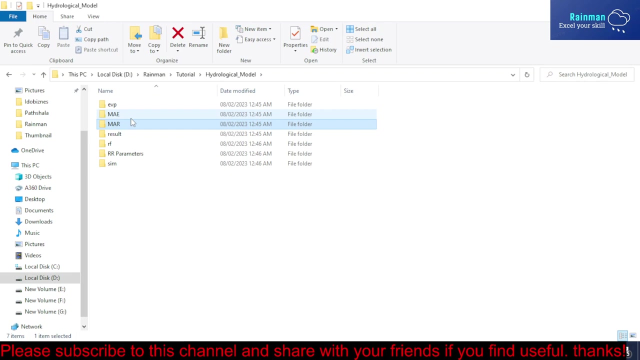 and another one is mar. these files will also be created when you run the model or when you calculate the basin area. it will be automatically generated. so nothing to do with this file. actually, these two folders will be empty, initially empty. when you run or simulate the model, this result file will be created automatically. mar stands for mineral rainfall. 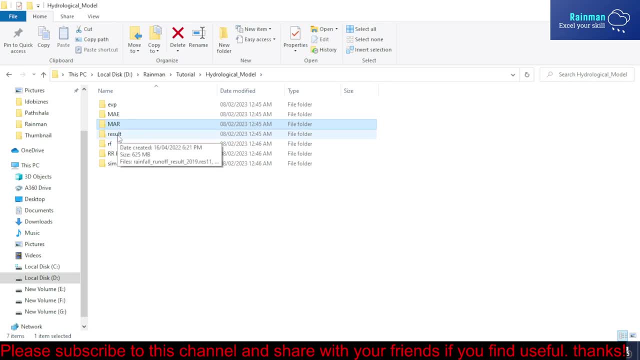 and and the fourth folder is result. in this folder your result file will be saved and you will show the directory in your simulation file in this result folder and the result file will be saved here during the simulation. and this is rainfall: the rainfall stations which govern your hydrological area. 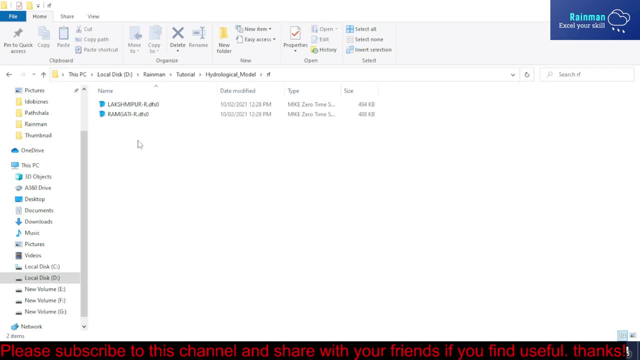 these stations data you have to place here in this location. suppose, for instance, in my hydrological area there are two rainfall stations. name looks me poor and ram gothic. there are two time series, individual transits. i have just. i've just put here another one. it is very important thing: rr parameter you have to. 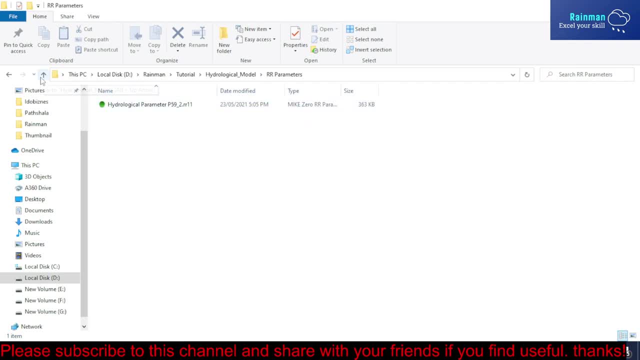 create a rr parameter file before simulating a hydrological model. rr parameter means rainfall runoff parameter files. this is the main thing. the main important file extension is rr11. you have to at first you have to create this rr1 file and then you have to place. 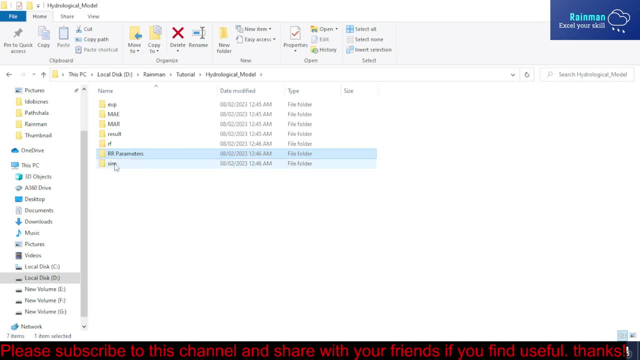 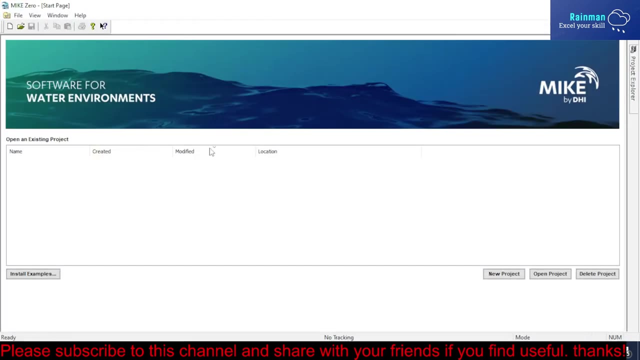 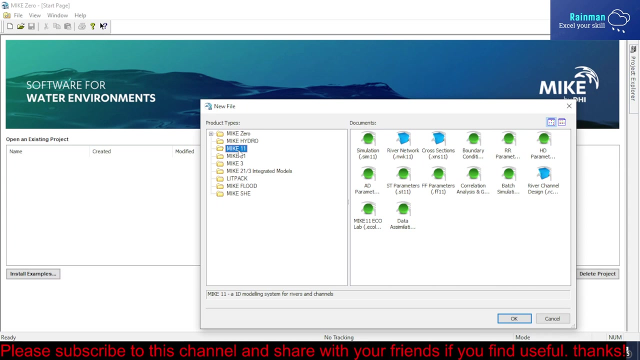 that rr1 file in this folder and the last of all, the same file theme folder. under same folder, you will keep the simulation file. so now let's see how to create rr parameter file. first of all, this is the rr parameter file. you have to create this rr parameter file and then click on new, then click on. 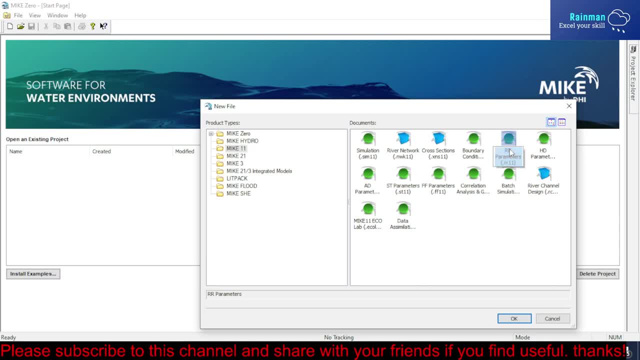 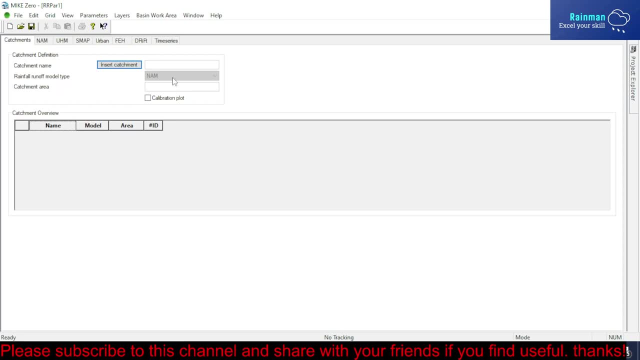 my one, one module. under this. there are some options. click on our parameter dot r r11 and double click on this is your rr parameter file. you have to prepare this file accordingly, according to your catchment characteristics, your uh, associated data, uh, which you're recording for your hydrological. 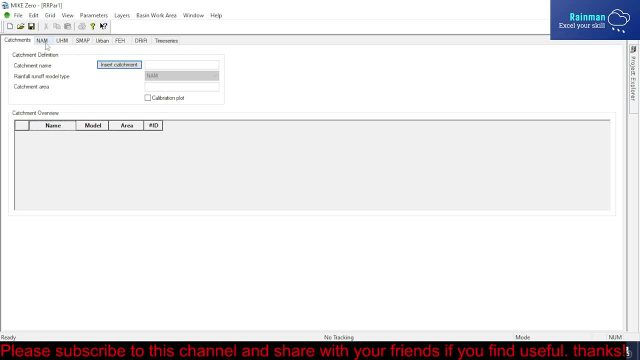 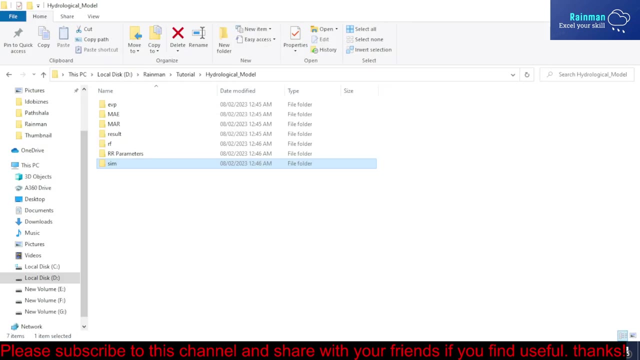 model. so under this rr parameter there are different kind of tabs like name, qhm, etc. etc. so i'm not doing any work on this file. i have a ready file. i'm gonna show that file for quick video. let's say, i have already prepared a rr parameter. i'm opening this parameter file. 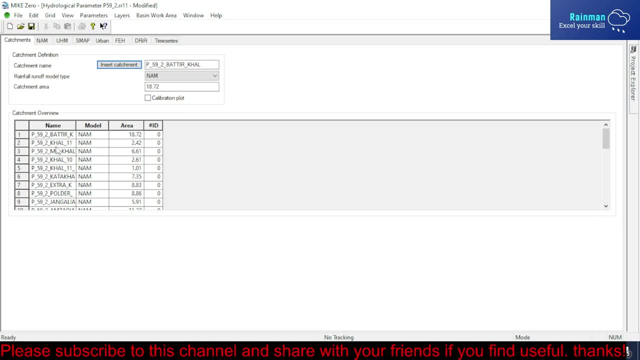 the first of all catchments. so this is actually a hydrological model of area um. area means a folder area. actually there are several calls. you know there are 33 calls in under that folder. the folder name is 59x2. oh so i digitized the catchment for each catchment. this is a catchment. 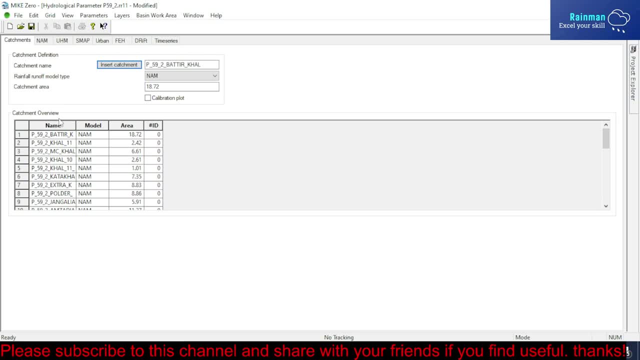 call and found out the area and prepare the catchment like this. catchment delineation is also important. what are the considerations for catchment? and that is that can be another video. if you know how to delineate catchment, then you have catchment area, you have corresponding in the 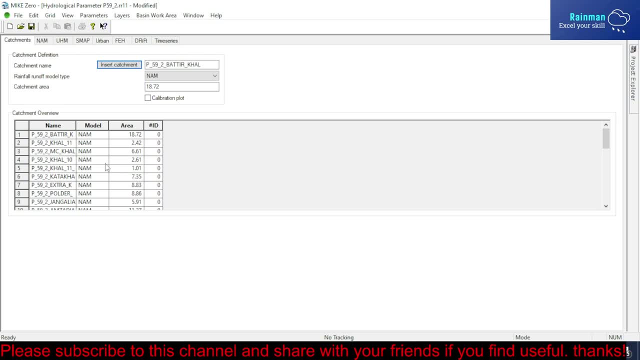 uh canal or river in that area. so this is the corresponding canal, the the corresponding area of that canal. i mean the catchment or watershed area of this canada is 872 kilometers square and, and similarly for all other calls, the catchment area is like this: if you want to add another catchment, then just click. 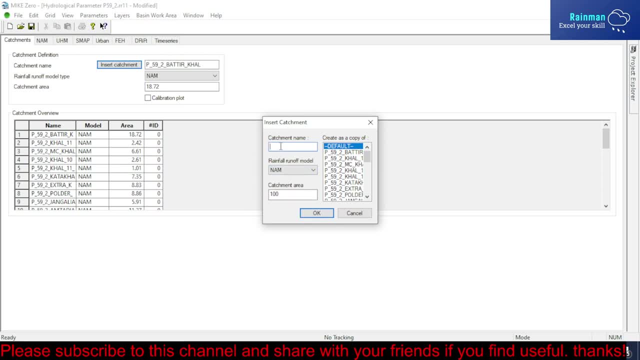 here: insert catchment, then you have to write the catchment name, then estimate area, then it will be added at the end of this table. so another way you can do it, just if you have the excel file, you have to insert the row and the code and then copy from the excel file. just paste here the all informations. 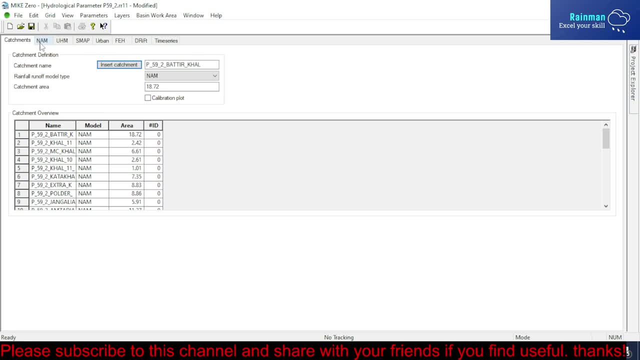 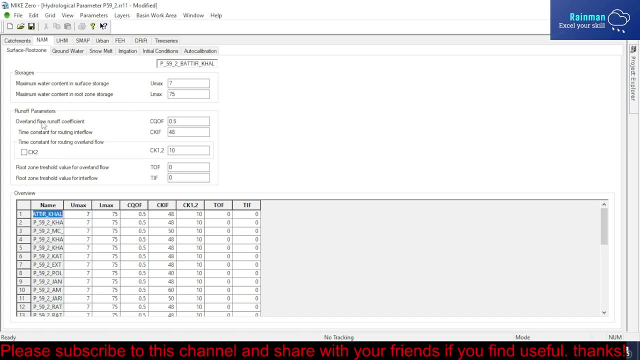 of catchment. then come to the second tab that is name. so you are seeing here so many parameters are here. so automatically for each uh channel or each color canal there will be some parameters. these are the maximum water content, surface storage, zone storage coefficient, time constant for routing flow, overland flow. these are the main. 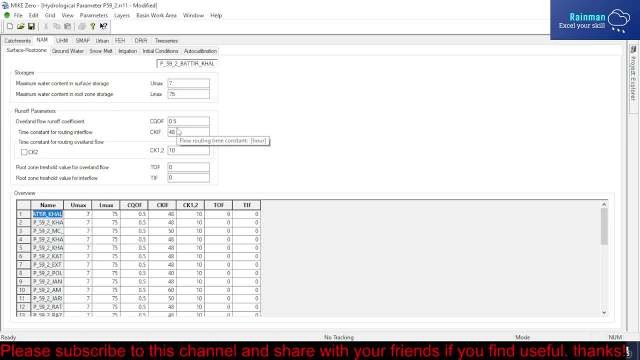 calibration parameters, actually by default, the values that will appear when you are gonna do it. you will keep this value after simulating. if you have measured value, you will change these values and calibrate your model with your measure. measure result: measured uh, measure discharge: what is the? 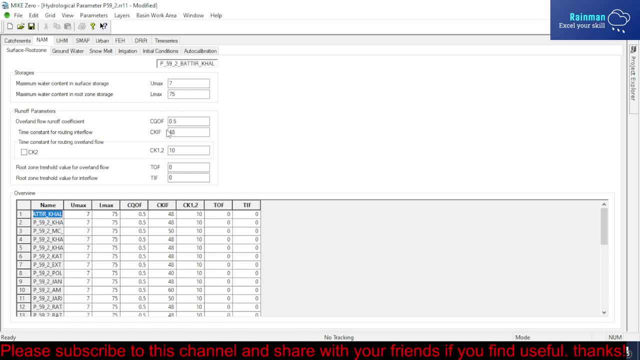 output of a hydrological model, you will get discharge right. so if you have a measured discharge of a outlet, you can compare your simulation model with your measured result. it will result with the measured discharge. if it doesn't- it doesn't match with you measured discharge- then you can change these values. or if you want to know that, what is surface? 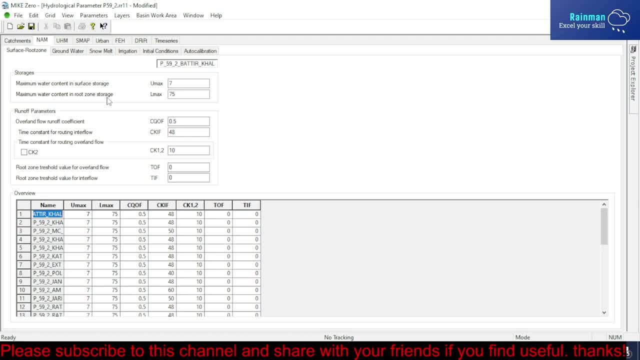 storage roots to road zone storage and storage. you can google it what it is actually. or if you are a student of civil engineering or water resources engineering background student, you must be knowing this terminology. i'm not going deep into it, but if you are a student of water resources engineering background student, you must be knowing this terminology. i'm not going deep. 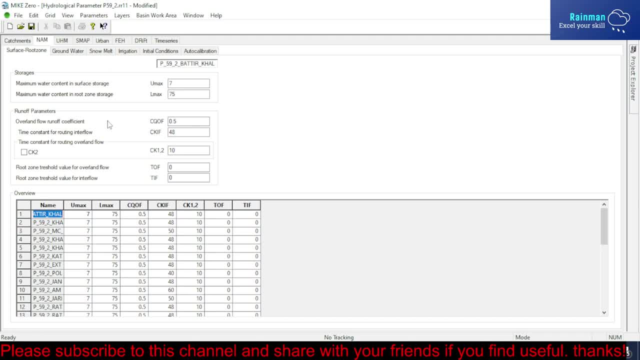 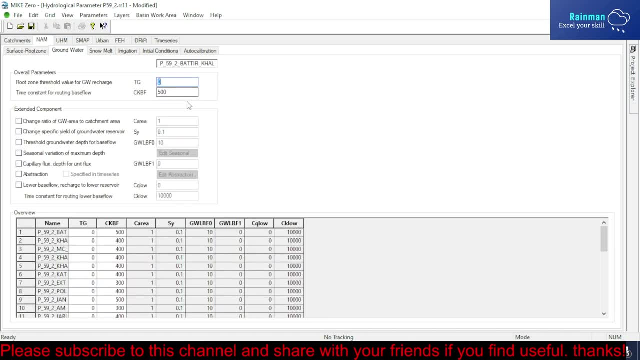 deep into this. this is the process. actually, by default, some values will come and then you have to calibrate by changing these values and similarly, this is the routing base: flow constant, time constant and ground water recharge constant road zones, threshold value. some default values will be appear and you will do it by default value. then, if you want to calibrate, 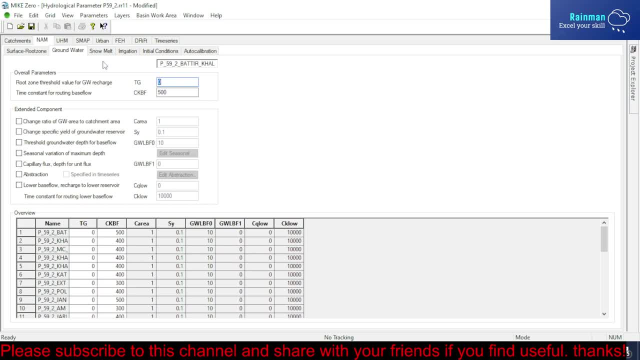 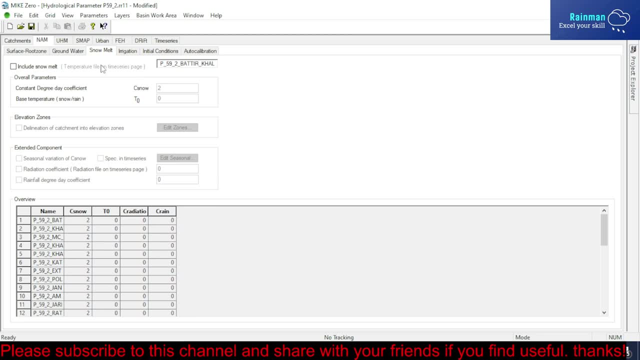 the model, then you have to change it. these are also the calibration parameter of your hydrological model. snow melt, snow melt. actually in bangladesh there is no snowfall, so we actually don't check mark it. if your country a experiences or faces no fall, then you can check mark it and, of course, and the corresponding value you can add, so irrigation, if you. 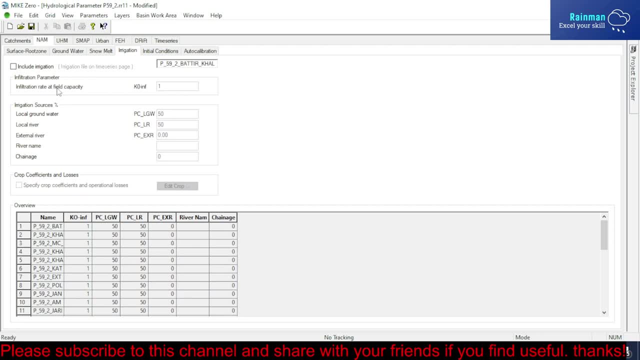 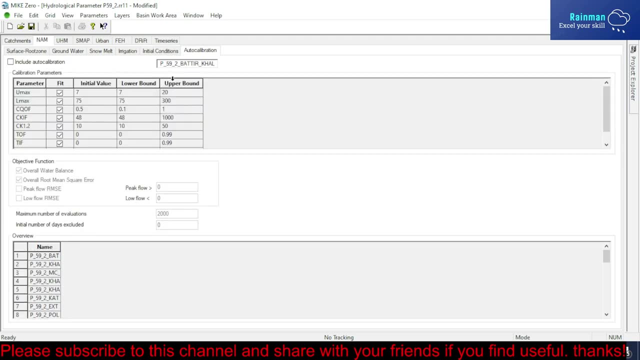 you want to include regression, then you can or otherwise. just uncheck it, no problem. initial condition as it is. you just keep it auto calibration. you can check mark it, then it will be auto calibrated or otherwise it will not auto calibrated. you will have to change the values. 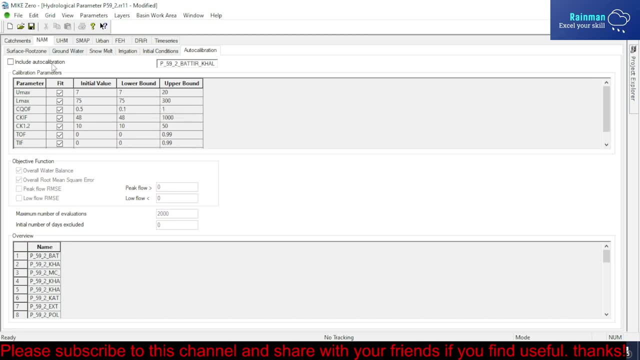 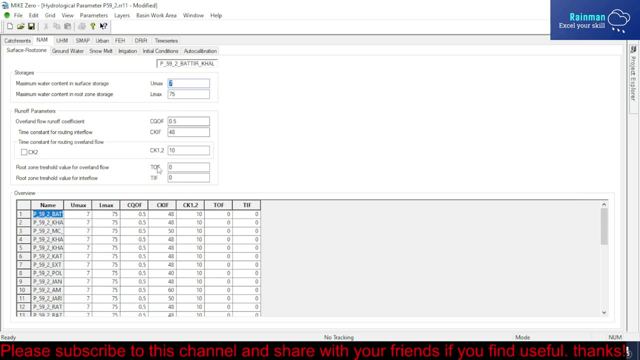 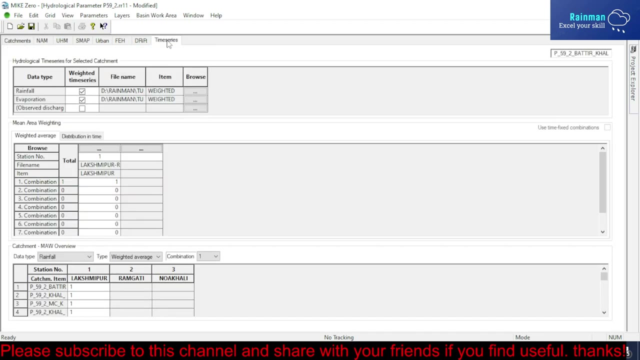 manually this umax lmax. umax lmax is the calibration parameter i have already mentioned before. these are the see. these are umax lmax. these are the thing now. the last of all. the last step is time series. so you have rainfall, time series and 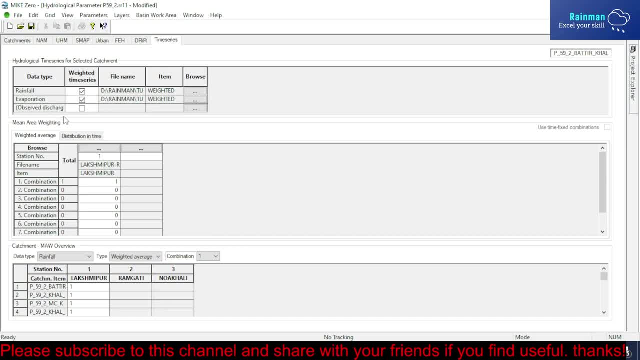 evaporation time series. these are the main data you can use for the time series. so you have rainfall time series and evaporation time series that you need to simulate a hydrological model. so first of all, data type. suppose rainfall i have. you have to show the 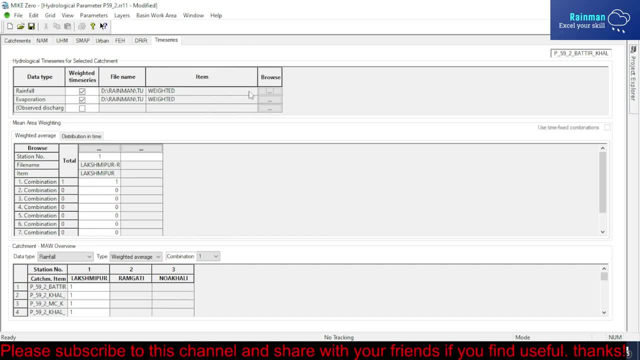 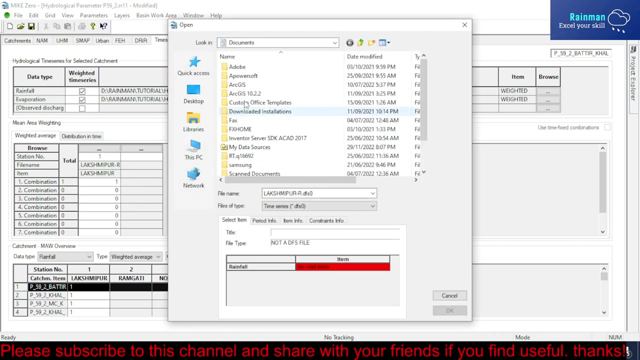 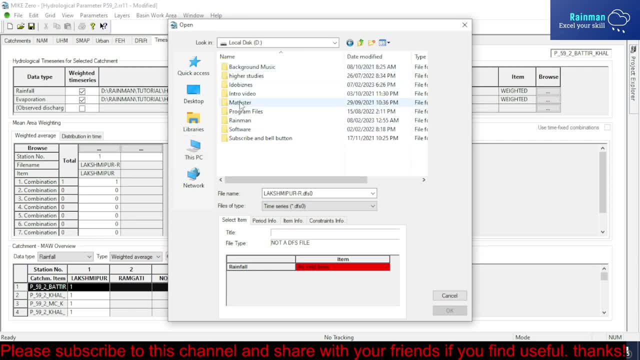 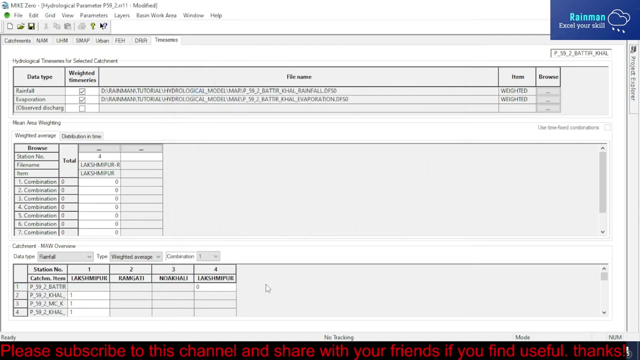 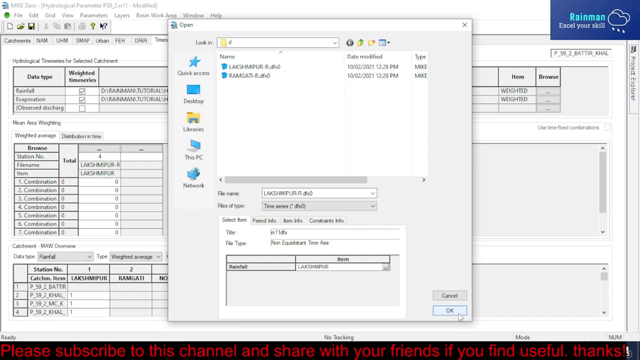 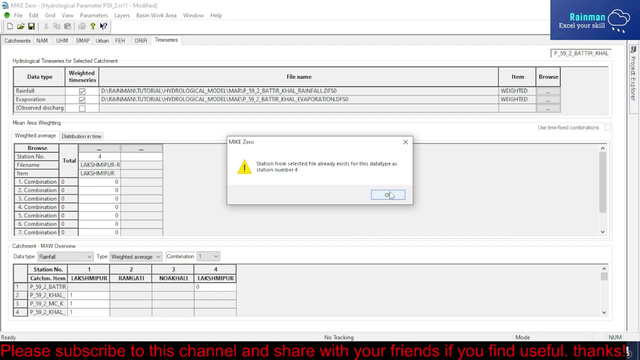 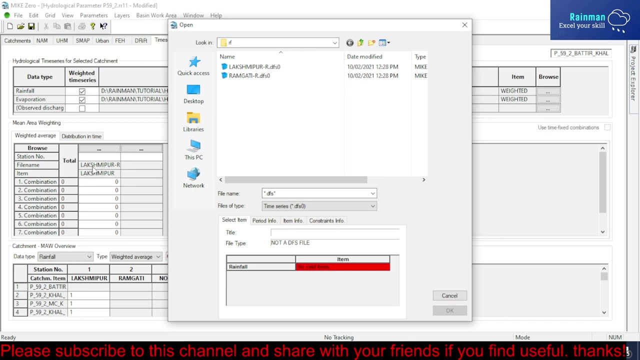 this one. okay, nice again there. there you can prepare several kinds of combination. these are the rainfall, so how many rainfall station you do have, you will set from here. break by clicking here. suppose you have already set the lakshmipur, then you add the ramgati. okay, so we have lakshmipur and ramgati. 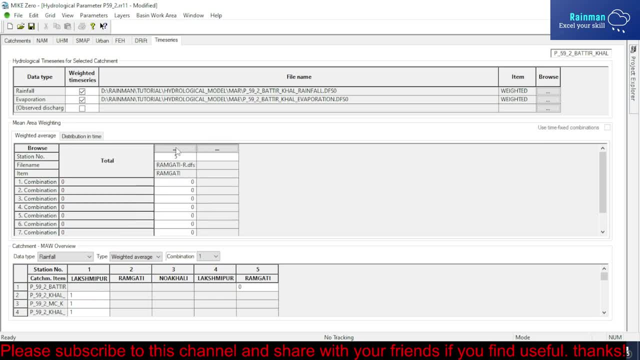 this five station. five is already there if i set it lakshmipur, okay, so you can see that it's already there, okay, okay, i'm. i'm just giving you as an example. i will use the previous one. i'm just showing you how to add the rainfall station and evaporation station so in every catchment you know the. 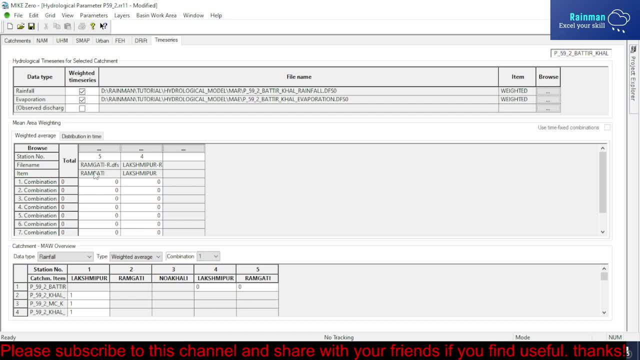 percentage of ramgati station uh influence and the lakshmipur uh station influence. so here five is ramgati. okay, so you will give your percentage. let's say it has forty percent and it has sixty percent contribution for catchment one or for this panel you have to set like this: 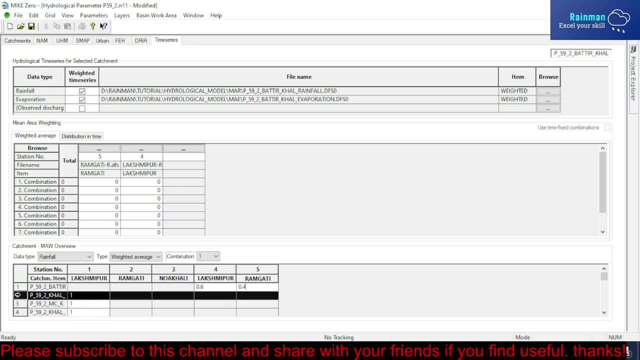 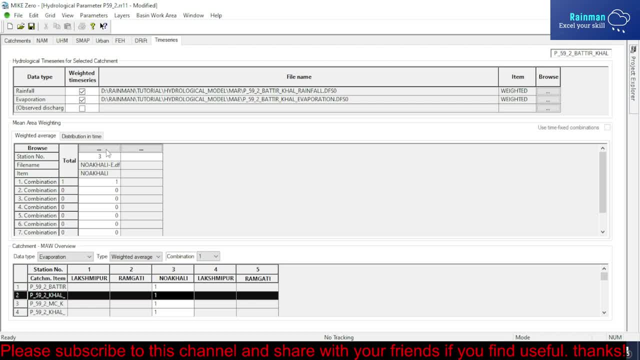 time series from your evaporation folder. and uh, let's say okay, um, Here you will give the 100% contribution of your operation station. you will set one for each catchment. here see, in every value there is value one, And for every catchment, suppose for one. 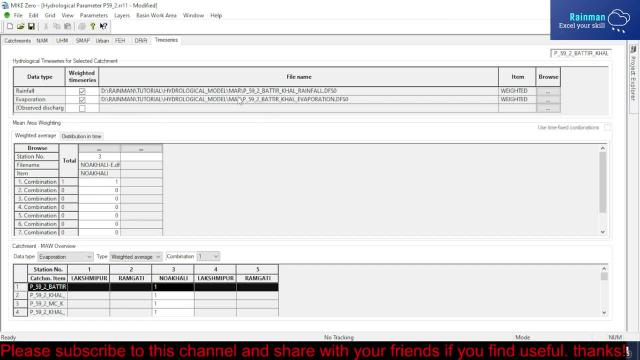 After providing this, you will set the folder here. the MAR, this is rainfall MAR And this one evaporation. you have to set MAE. After setting for each call, you will click on basin work area. Calculate mean precipitation. you will click here. 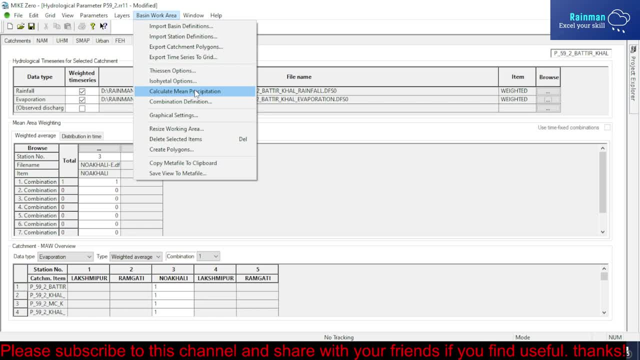 In the previous version you must click here before simulating the hydrological model, But in the latest version you don't have to click on the click calculate mean precipitation when you start simulating then it will be automatically created the associated files, the rainfalls that I have shown in the MAR folder and MAE folder. 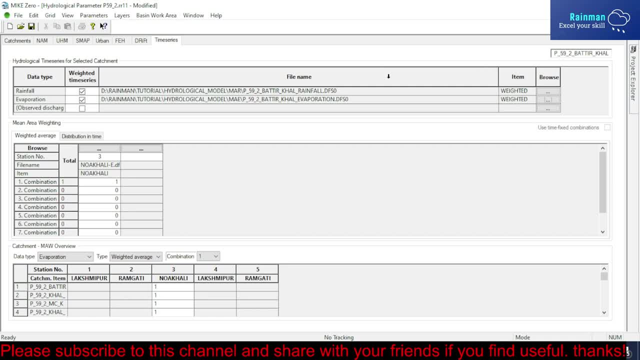 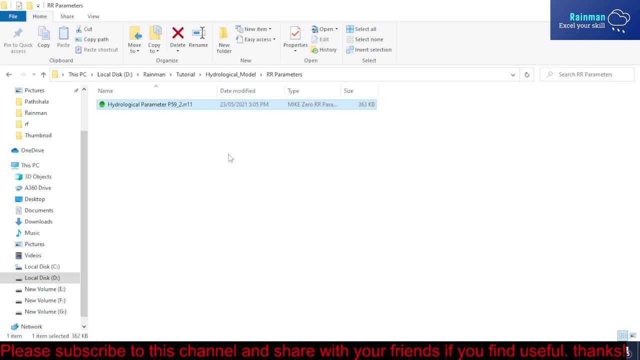 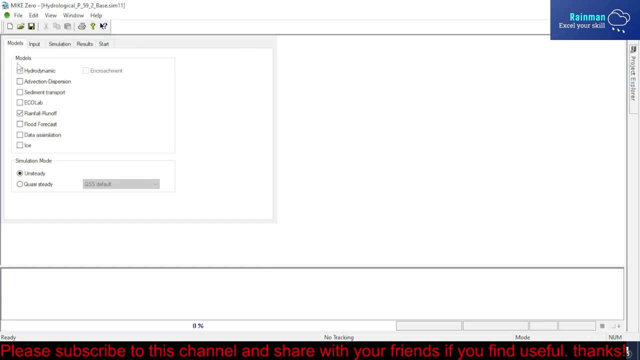 It will be created automatically. I'm not going to do this and I will not save this. Let me show you now the sim file: the setup of hydrological model. This is the sim file of name model. Actually, how will you do it? 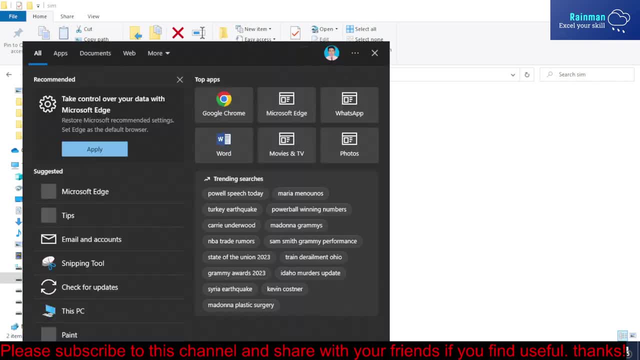 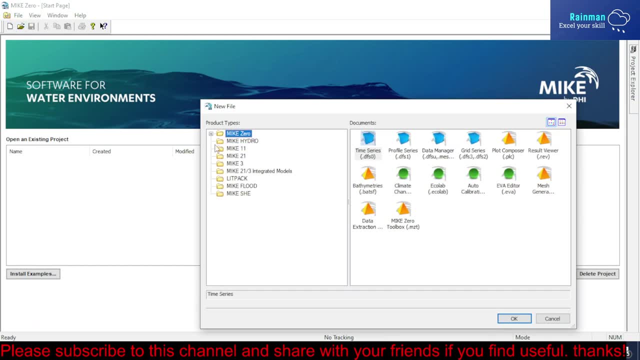 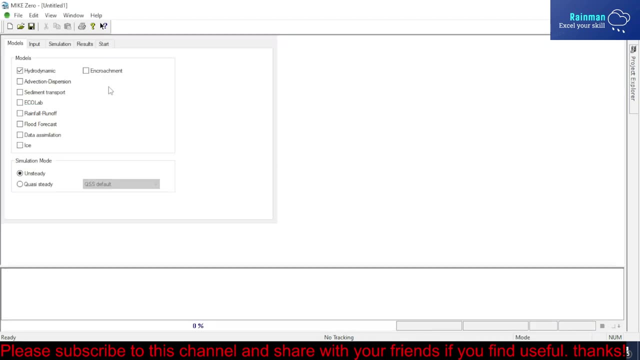 When you open, Let's say, Mike zero, When you open the Mike zero interface, then click a new, then click on Mike one, one, And here you will see the simulation sim one. Then this is the main interface of you know the name. 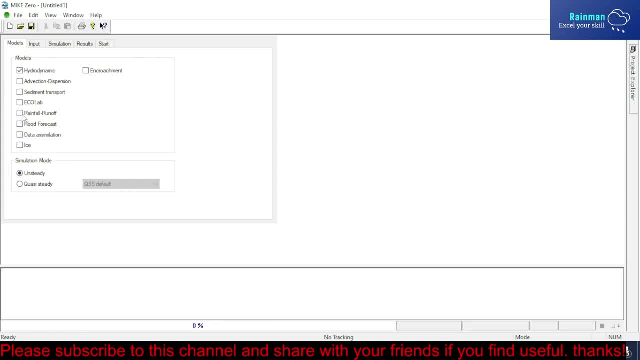 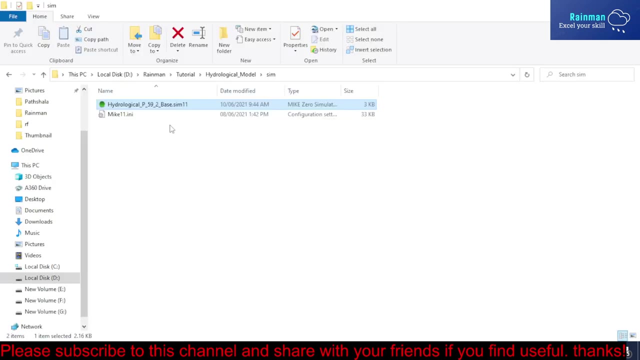 If you want to run the rainfall runoff model- that is, hydrological model or name model- you have to check market On. you have to check it on. That's how you will open the theme file. So I am just opening my previous theme file. 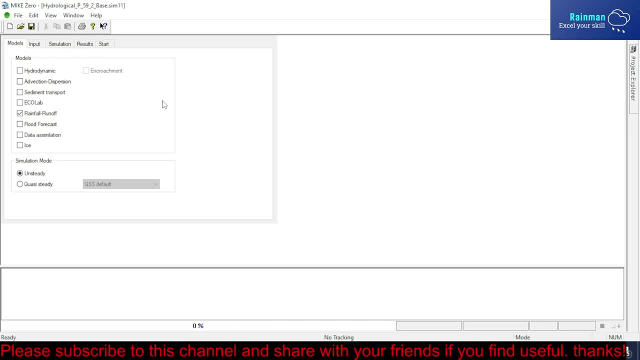 Then I'm going to do you the step by step method: how to set up the sim file. First of all, check mark on the rainfall runoff model. The simulation mode is unsteady. The input, what will be? the input input will be only the rr parameter file. so from here, 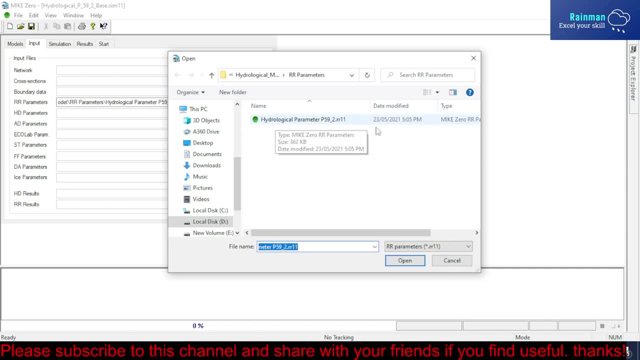 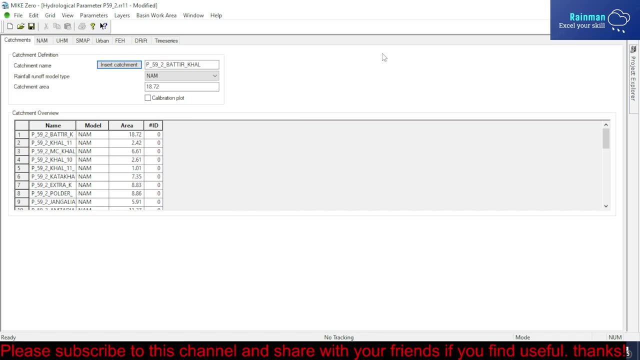 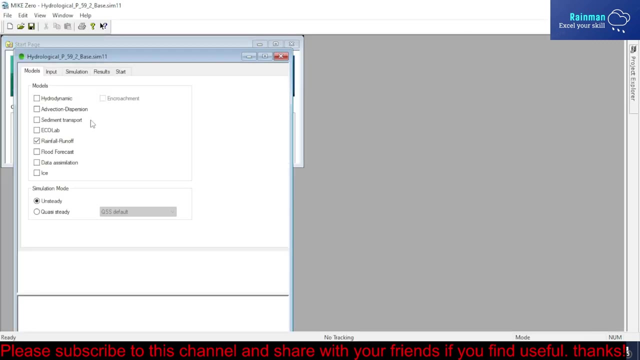 you can add your rr parameter that you have just created and add here, and you can edit your rr parameter file by clicking here. okay, then come to the simulation. uh, time step type: give fixed time steps. type: usually provide fixed time step and let the time step five minutes. 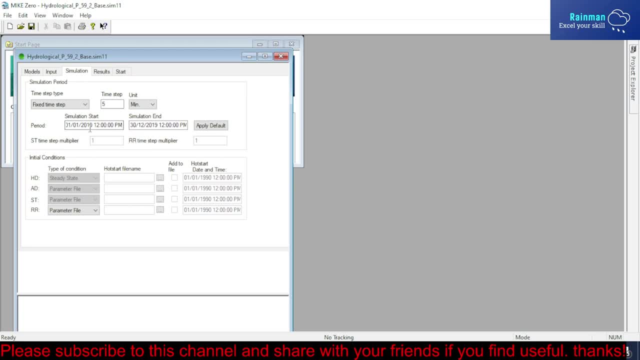 every five minutes the calculation will be done and the simulation start and simulation end, in which, for which period you want to simulate the model. you have to provide the data correctly here or apply default. if you provide applied default rainfall, rainfall or evaporation time series that you provided in the folder rainfall or evaporation. 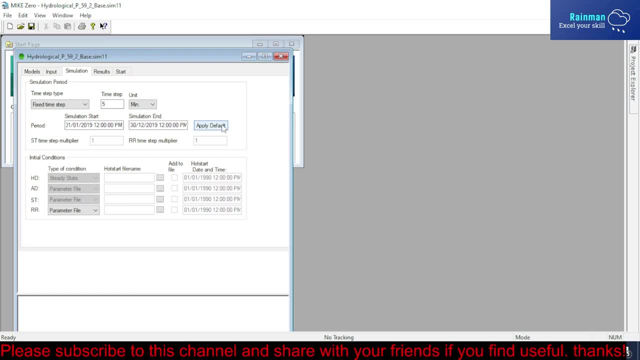 folder accordingly, according to that time period or your, according to your data set, it will be set automatically. otherwise, if you have, if you have a desired time period, then you have to the time period manually. so, rr, here you have to provide parameter file, then result, and rr: this is rainfall runoff. 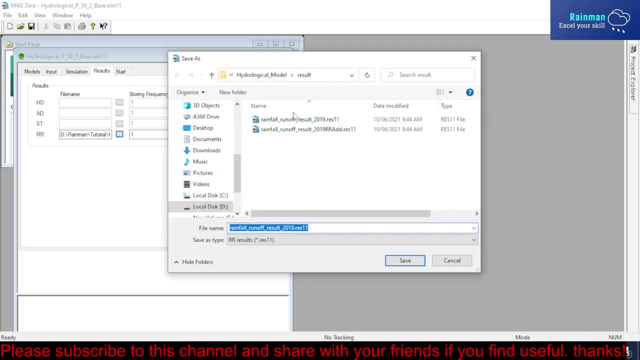 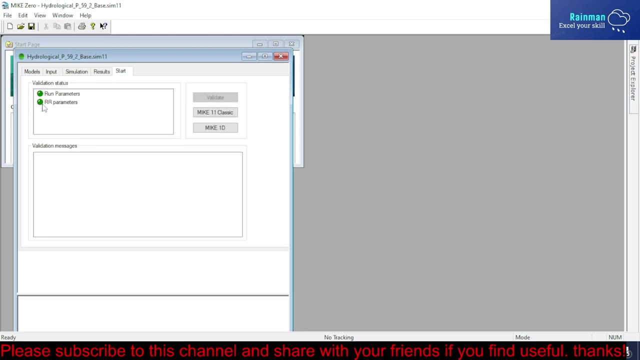 you have to show your result folder. this result folder you have to show here or you have to, you know name. you have to write the uh, your your result file and say you'll keep the same. then start, if you see the two green dot here: run parameters and rr parameters. 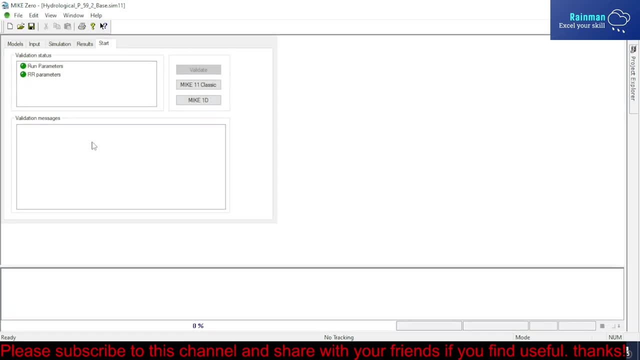 so it is okay for your simulation. your setup is ready and once your setup is ready, you can go for simulation. then click on mic 11 classic, then it will uh simulate your model and give you the result. so let's start. so click on this. i'm not clicking on this because my result by previous result file. 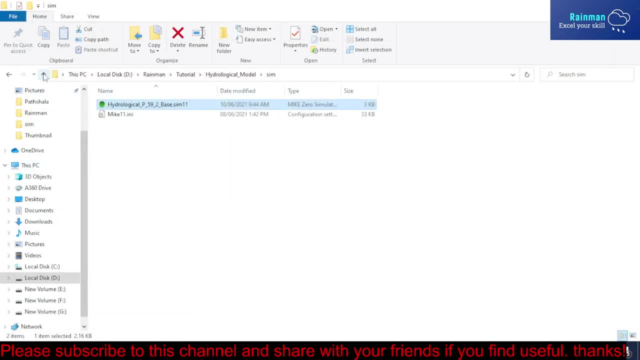 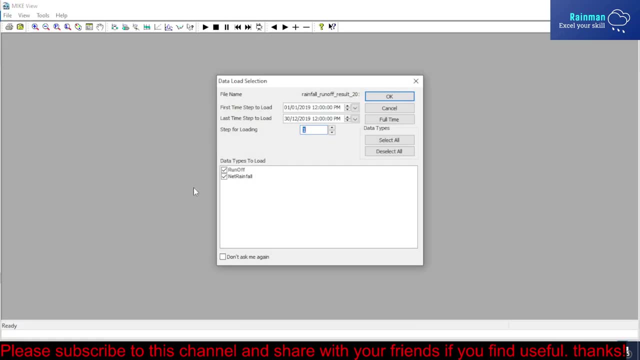 will be deleted if i click this now show. let me show you the result file directly. this is result. this is my result file. see, we have uh runoff and net rainfall, so our main output is see the runoff. You can see the runoff for each catchment: Click on. 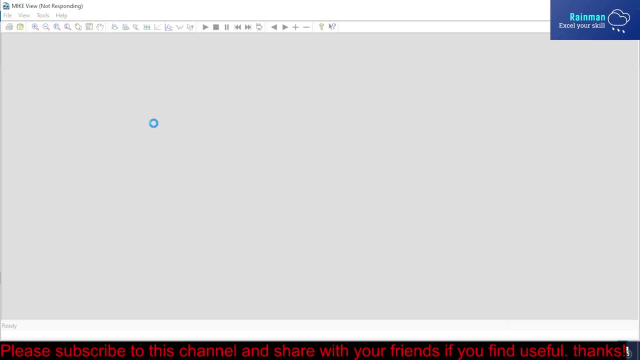 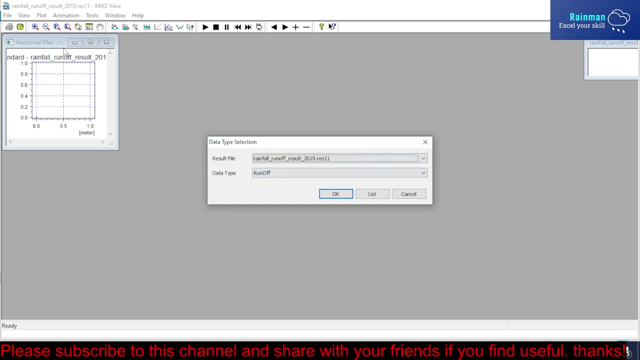 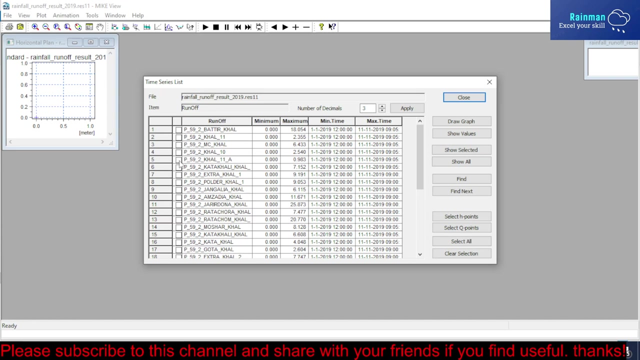 Oh, sorry it's not responding because of my laptop technical issue. My result file has been just opened. So this is my rainfall runoff result. Data type here: runoff. Now see the list. So see all the channels, all the calls, all the channels in your catch, in your area, in your model area are listed.